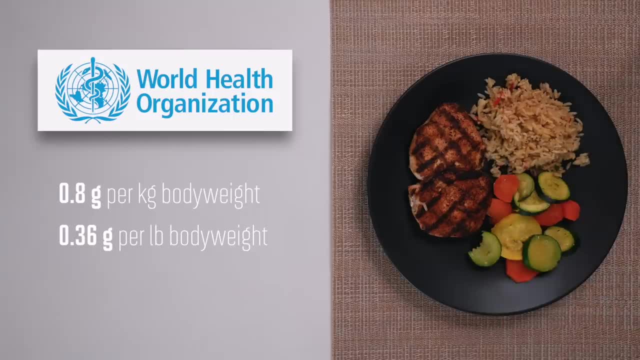 protein per kilogram of body weight or 0.36 grams per pound. So an 80 kilo or roughly 100 grams of protein per pound of body weight. So that's a lot of protein. So I'm going to pound. person would only need about 65 grams of protein per day. This is pretty hard to miss on a. 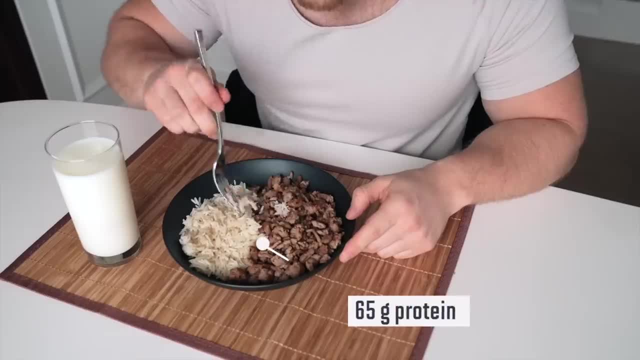 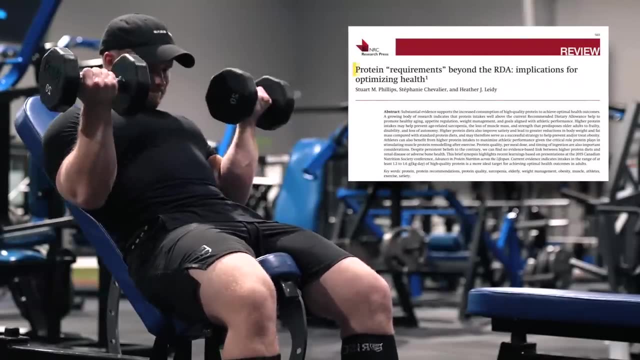 typical Western diet- I mean this ground turkey- and rice bowl with a glass of milk- has 65 grams of protein and that would have me covered for the day. However, this recommendation doesn't consider weight training and many protein experts have called for an increase, given the abundance. 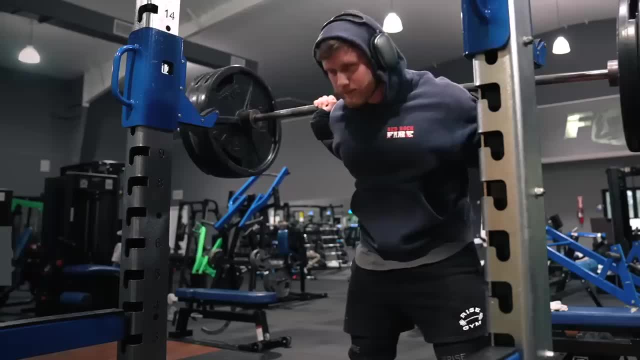 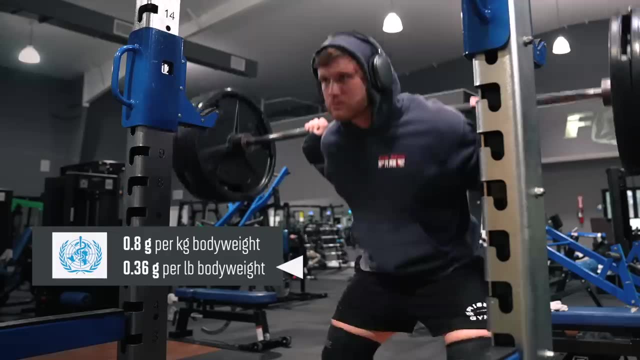 of evidence showing health benefits with higher protein intakes, And the sports nutrition research is perfectly clear in showing that this amount of protein simply won't be enough to support, much less maximize, muscle growth. For that goal, we'll need more. Now just how much you need. 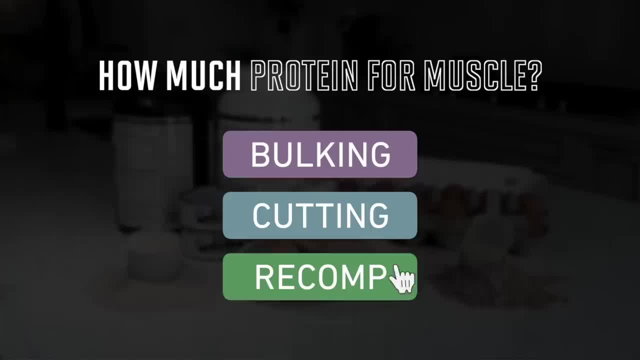 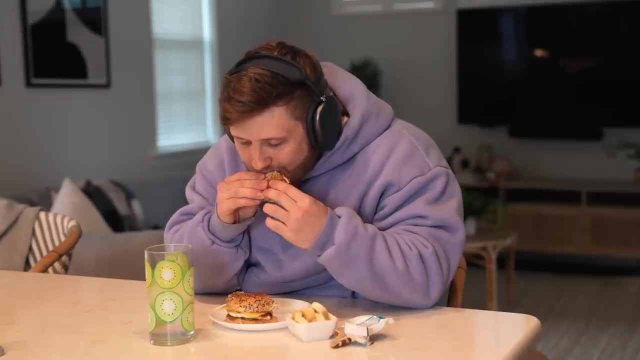 depends on if you're bulking, cutting or doing a recomp phase, And these ranges apply to both men and women. If you're bulking, your body is well-fed, meaning it's much less likely to break down muscle tissue as a fuel source. There are plenty of carbs and fats to burn first For this. 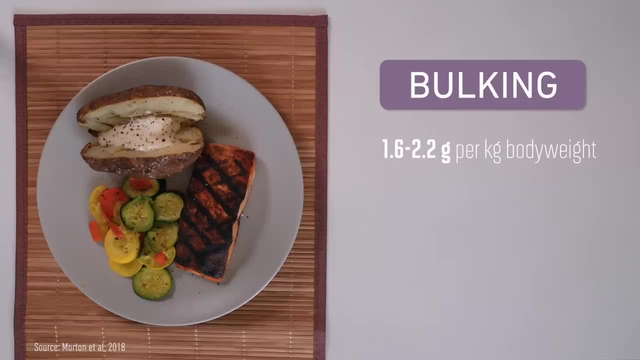 reason you generally need less protein when bulking. Here the best research recommends 1.6 to 2.2 grams per kilo, or 0.7 to 1 gram per pound per day. And here we can see the trusty old 1 gram per pound rule holding up pretty well as a high-end. 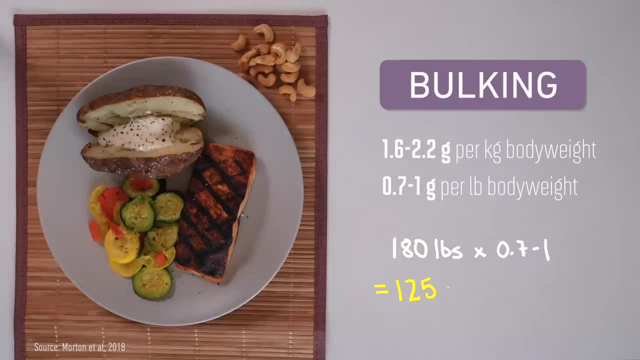 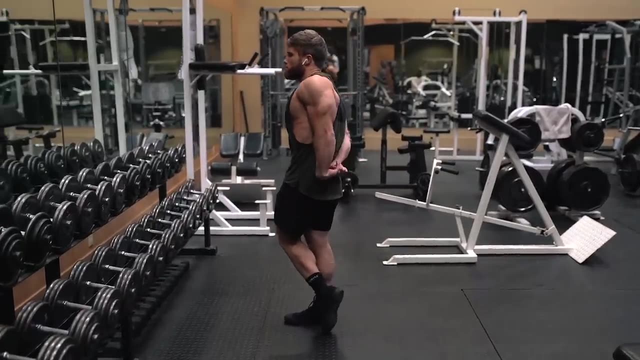 figure. So if you weigh 180 pounds or 80 kilos, you'd want something between 125 and 180 grams of protein per day when bulking. On the other hand, if you're cutting, your body's not only getting fewer calories from food, you'll also have less body fat and less glycogen as fuel. 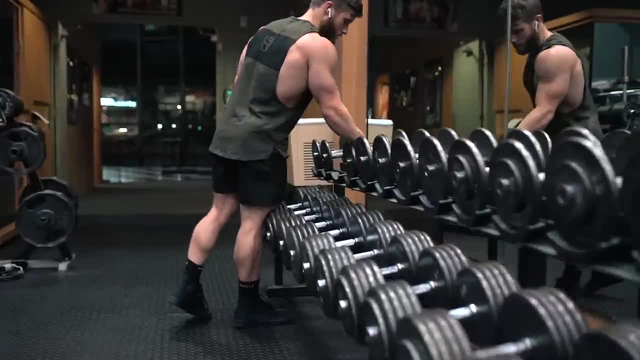 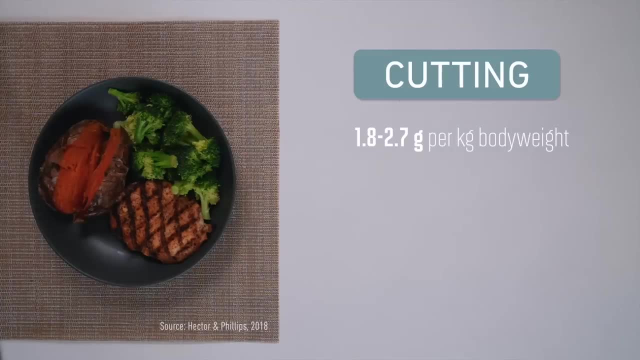 reserves. Therefore, your body is much more likely to break down muscle tissue as a source of calories. To offset this, the best data suggests increasing protein intake, while cutting to 1.8 to 2.7 grams per kilo, or 0.8 to 1.2 grams per pound, And this time we can see that the 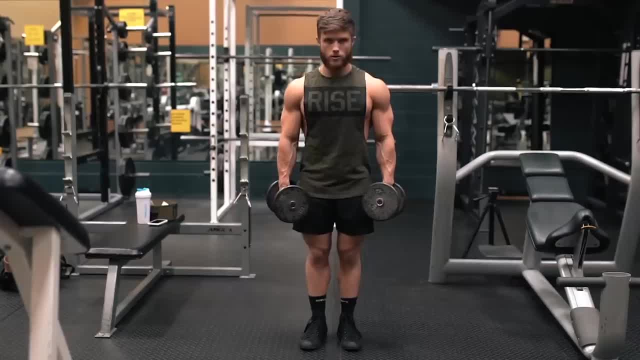 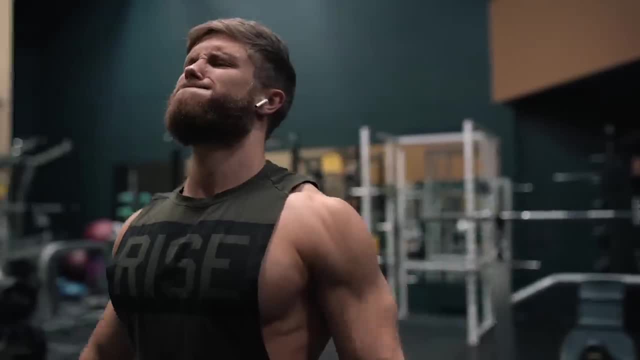 classic 1 gram per pound rule sits in the middle of the range. If you're already very lean and training very hard, you'll want to err toward the upper end, And if you have more body fat and are training more recreationally, the lower end will be plenty. Thirdly, when on a recomp phase, 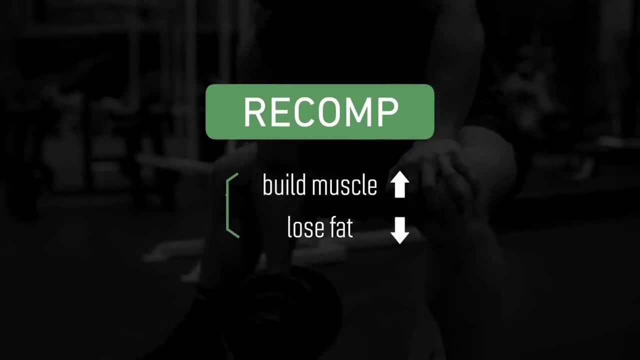 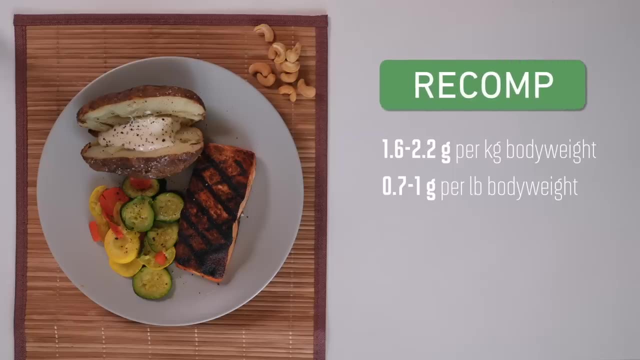 you're trying to build muscle and lose fat at the same time, while setting your calories around maintenance intake. So I think most people can simply use the same protein figure to build more muscle as when bulking, because at maintenance you're also at a low risk of muscle loss as long 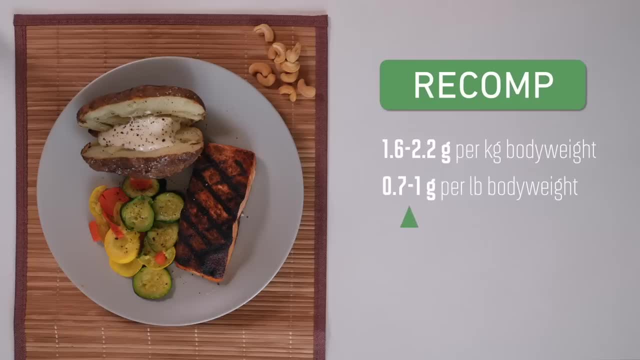 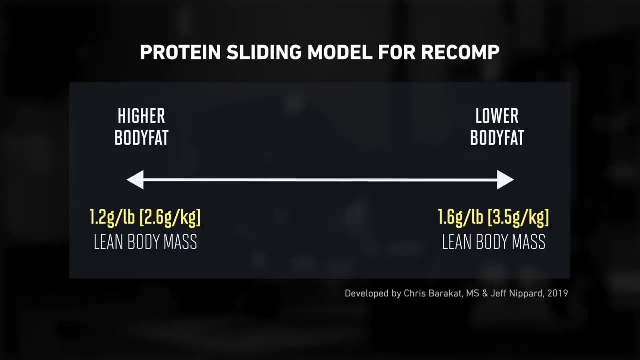 as your training is on point. However, there may be some advantages to going a bit higher on a recomp phase, especially if you're in a slight deficit or more advanced. In the past, I've used this sliding model as a guide for recomp, because it uses lean body mass instead of total body weight. 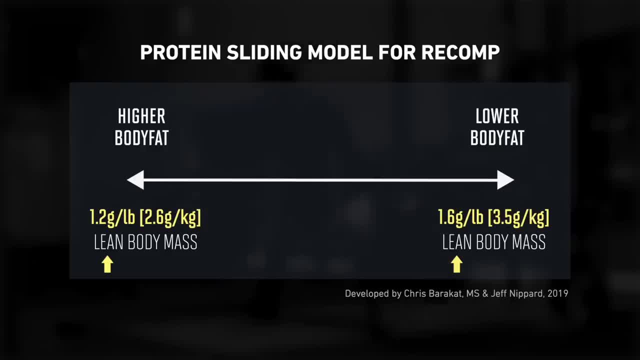 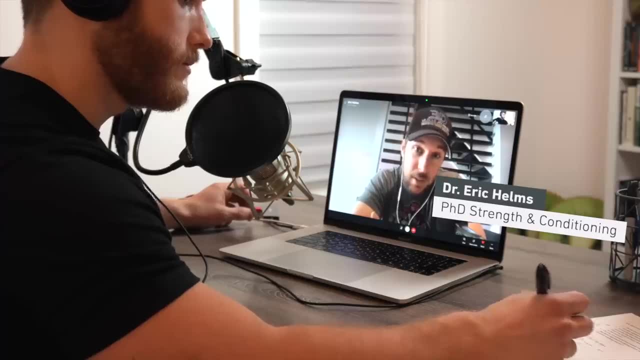 making it more individualized, especially for those who hold more body fat. However, the extra step of subtracting your body fat did confuse some people, so these days, I've come up with a simpler way to do this. If you're overweight or obese, you can simply aim for one gram of protein per 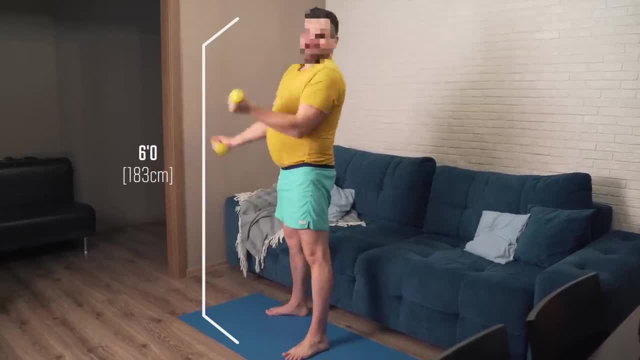 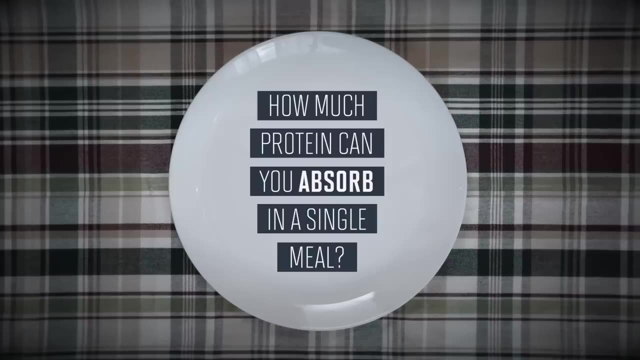 centimeter in height. So if you're six foot or 183 centimeters tall, you'd want around 183 grams of protein. This works shockingly well, especially if you're at a higher body fat. The answer to the question: how much protein can you absorb in a single meal is: all of it Your body can absorb. 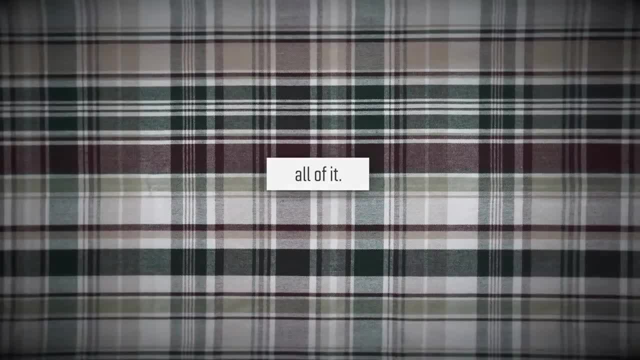 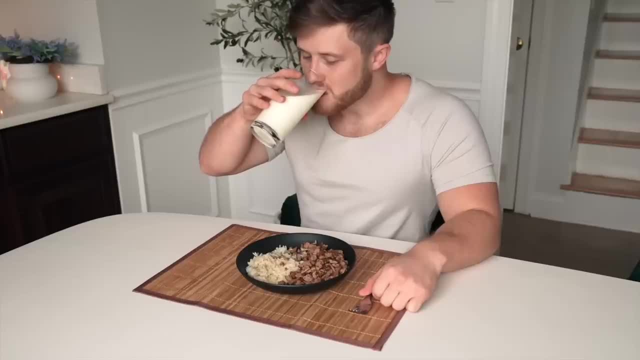 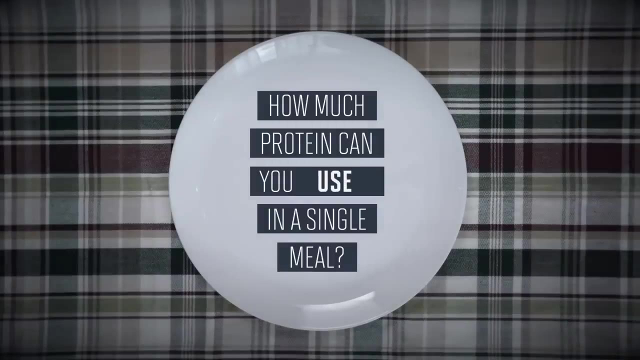 an enormous amount of protein in a single meal, more than you could even comfortably eat. But absorption simply refers to the passage of nutrients from the small intestine into the bloodstream. Just because protein is being absorbed doesn't mean it's being used to build muscle. So the real question is: how much protein can you use in a single meal? And this 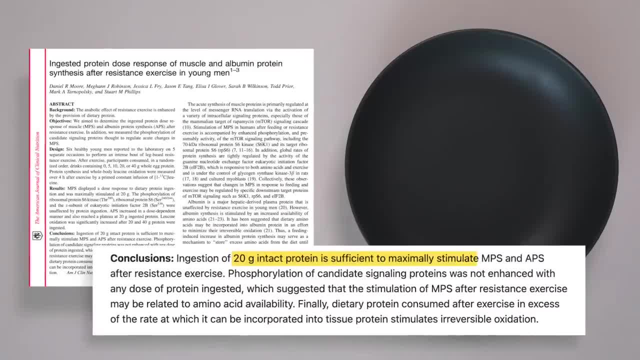 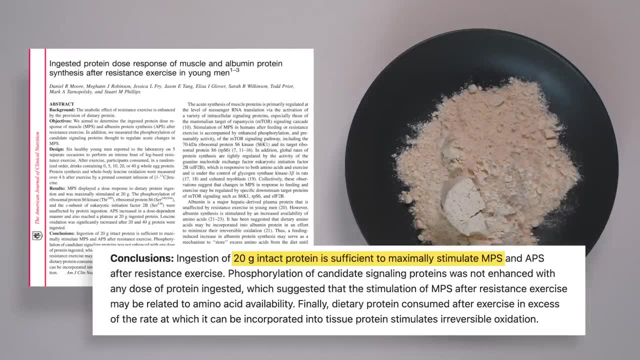 is where there's some controversy. The earliest research suggested that 20 to 25 grams of protein in a single meal was all you needed to max out the anabolic response, and going above that didn't do anything extra for muscle growth. However, I'm skeptical of this figure. First, on the anecdotal: 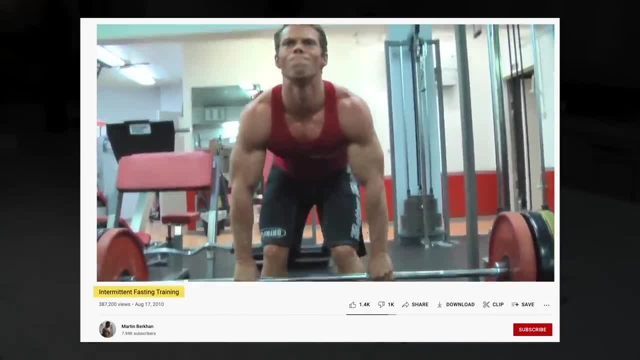 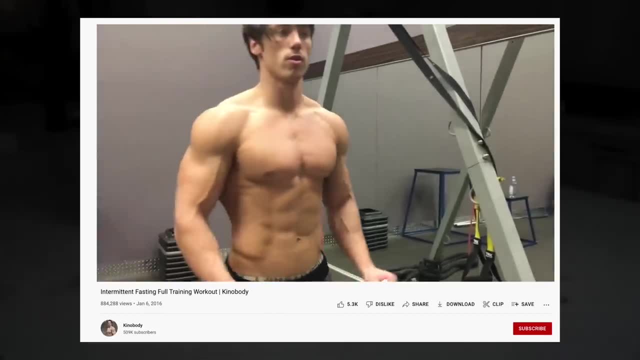 side there's a huge intermittent fasting community who seem to be getting plenty jacked from just one or two meals per day with upwards of 50 to 100 grams of protein per meal. It does seem unlikely to me, given their muscularity, that most of that protein is going to waste for these folks. Second, 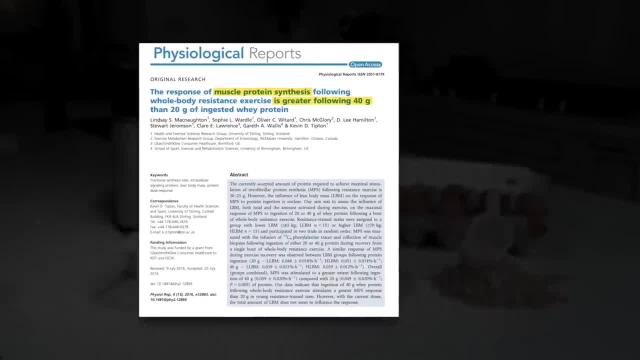 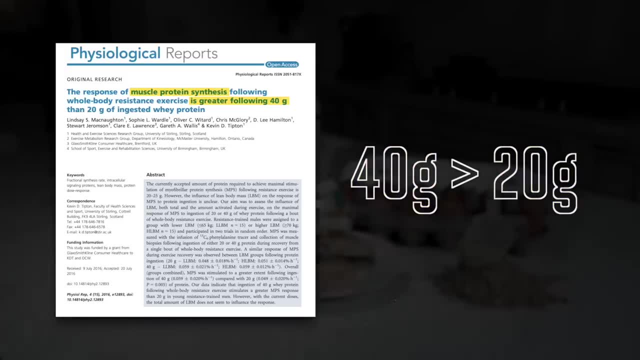 more recent research has challenged the idea of a 20 to 25 gram upper limit. This 2016 study showed higher muscle protein synthesis with 40 grams of whey, versus 20 grams of whey after a full body workout. and this 2016 study showed greater muscle protein synthesis from a meal of beef containing 70 grams of protein versus 35 grams of protein. So if you're a muscle protein enthusiast, you should be aware of this. So the amount of protein we can use per meal isn't clear as of now, but it's likely higher than we used to think And, regardless, I think that your protein intake per meal is. 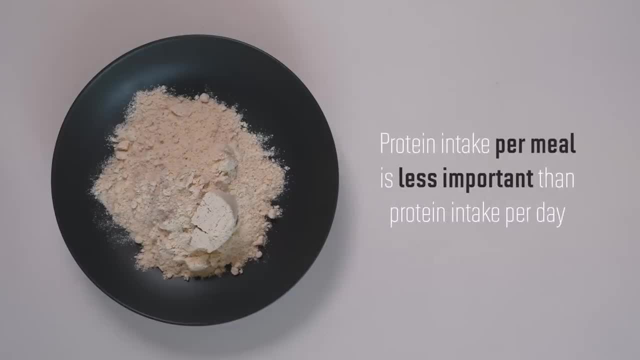 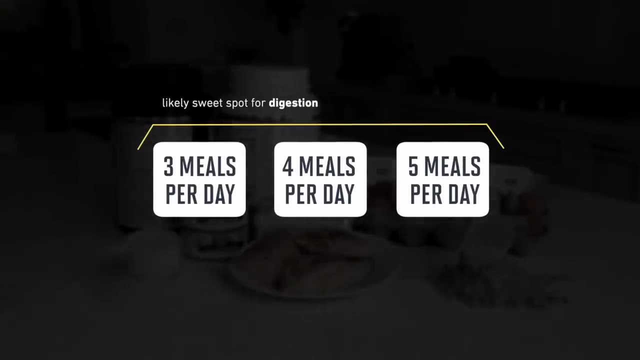 clearly much less important than your protein intake per day. Now, despite this, most experts do still suggest that spreading your protein out across three to five meals is likely best from both a digestion standpoint and for keeping muscle protein synthesis high throughout the day. Still, 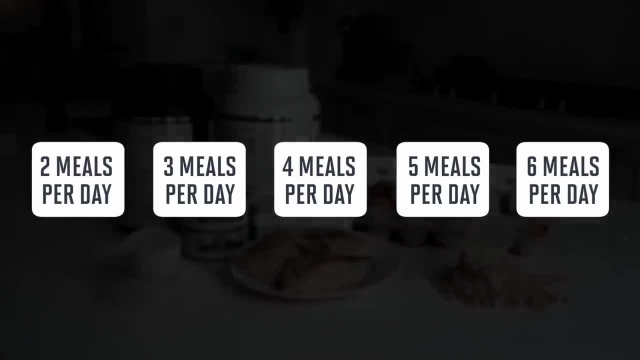 if you were to eat two meals or six meals instead, you will still build muscle as long as you're hitting your daily protein target, and if you're a muscle protein enthusiast, you're going to need a lot of protein. I just suspect it might not be quite as optimal. Protein quality is partly based. 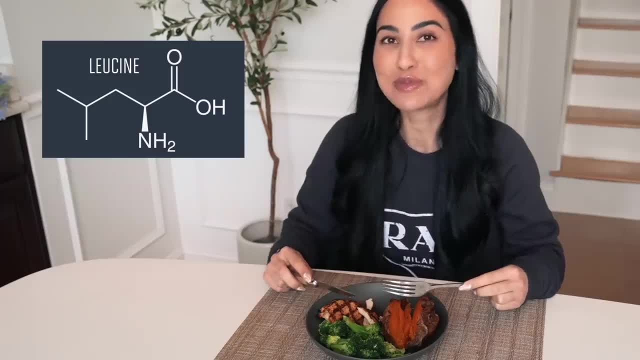 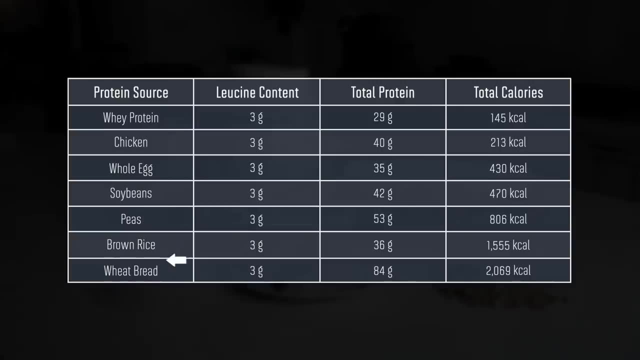 on the amount of the amino acid leucine. Leucine is very important because it is the so-called trigger for stimulating mTOR, which then triggers new muscle growth. So let's take a look at how much of different protein sources you need to eat to hit three grams of leucine, which is a decent. 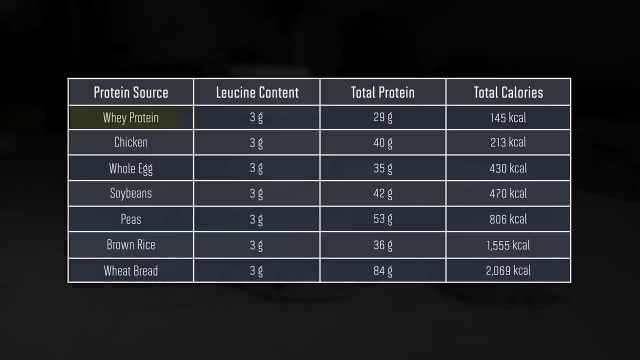 ballpark figure for maximizing the anabolic response to a meal. So in the table here you can see that whey protein comes out on top. In just 29 grams of whey protein you'll be getting three to 145 calories. You can also get three grams of leucine and 40 grams of protein from chicken. 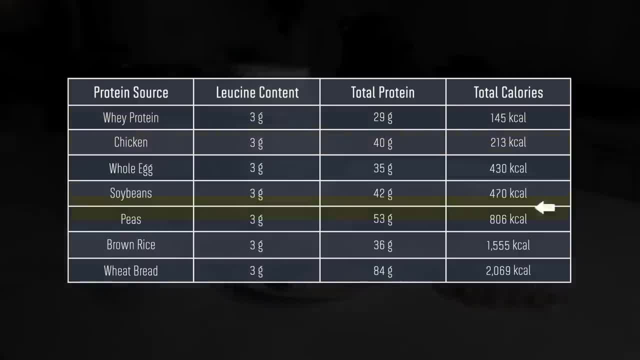 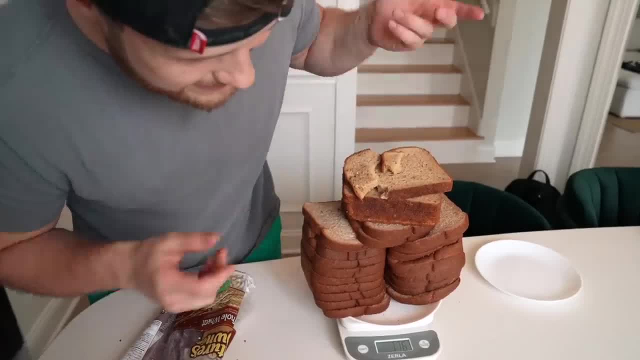 breast and that would only cost you about 200 calories. Moving down the list here, you can see that you'd need to eat over 2,000 calories worth of whole wheat bread to hit three grams of leucine. So it would take this much bread to give you the same anabolic punch as this scoop of whey protein. 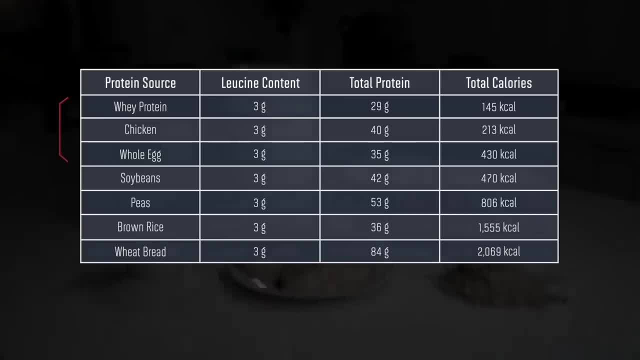 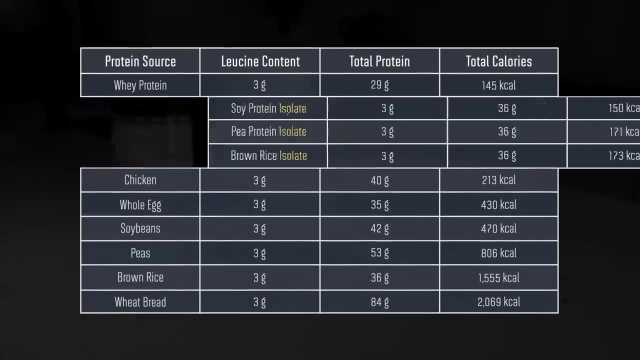 powder And, as a general trend, animal sources of protein are higher in leucine than their plant-based counterparts, especially per calorie. However, this issue nearly goes away once we get to vegan protein powders like soy pea and brown rice isolates, which also offer three grams. 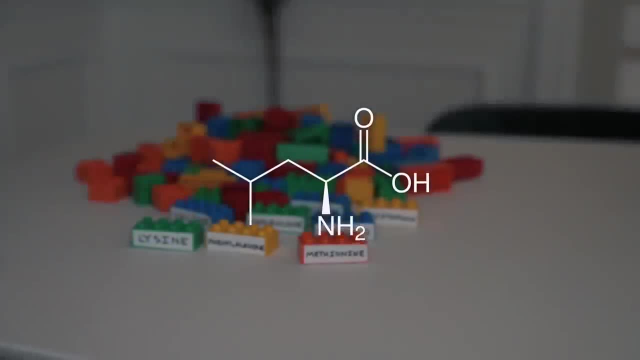 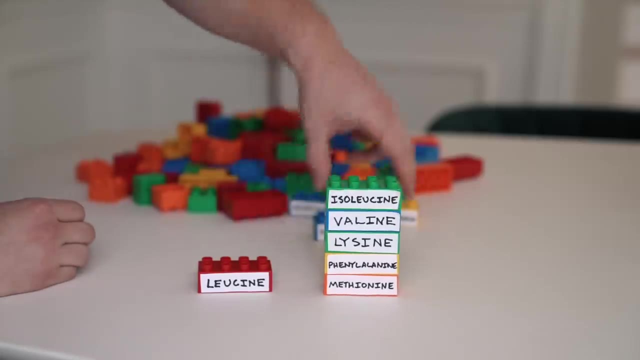 of leucine for less than 200 calories. But leucine isn't the only factor that matters for protein quality, because even though leucine will always spark the new muscle growth, you still need the other eight essential amino acids, or EAAs, to actually build the new muscle. For EAAs we use: 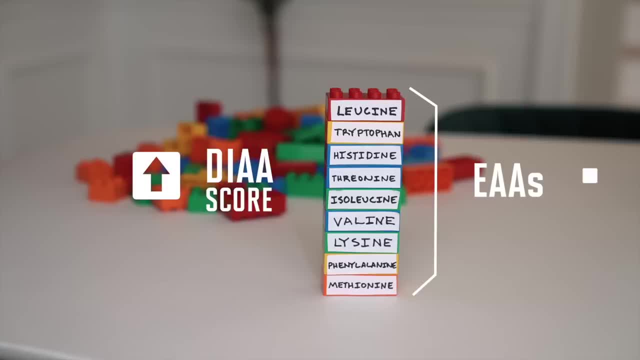 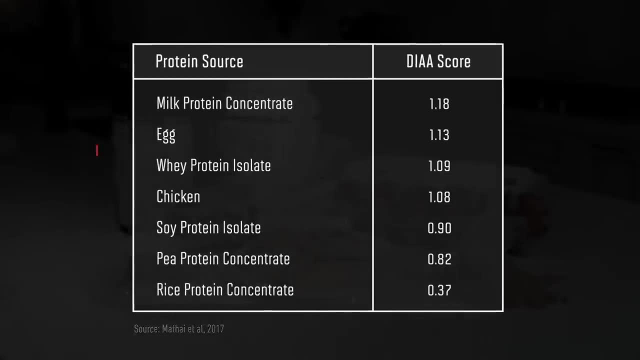 something called the DIAA score, where the higher the number, the more EAAs that are in that protein source. Once again, you can see that dairy and animal proteins come out on top. But a very important caveat is that these tables all refer to proteins being eaten in isolation In 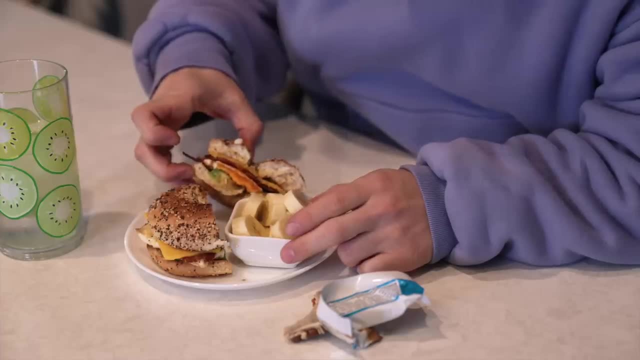 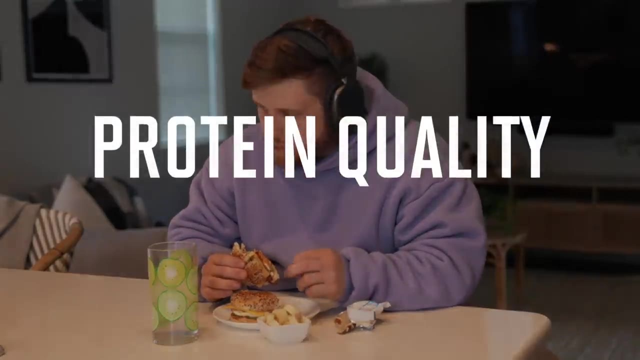 the real world. people combine various different foods and are almost guaranteed to get enough leucine and enough EAAs by simply getting enough total daily protein. So this isn't something I personally nitpick over, and it's why I think protein quality is actually much less important. 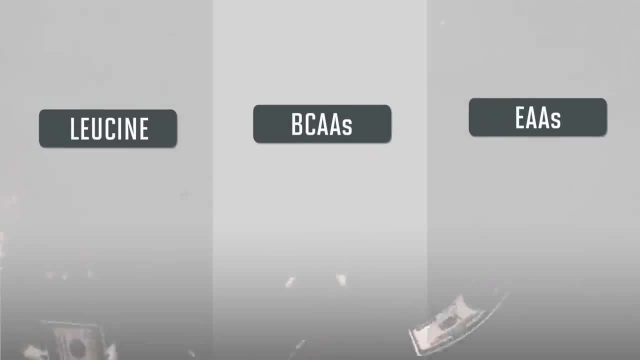 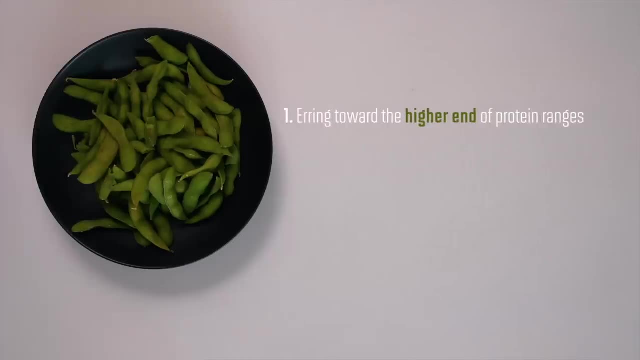 than many people realize. It's also why leucine, BCAA and EAA supplementation usually isn't necessary, as long as total daily protein is sufficient. However, vegan lifters should be a little more strategic by either erring toward the higher end of protein ranges and or supplementing. 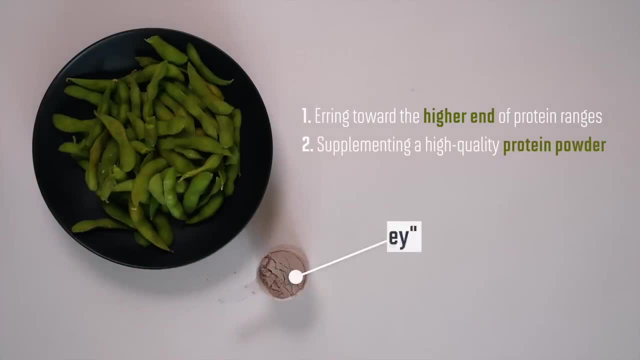 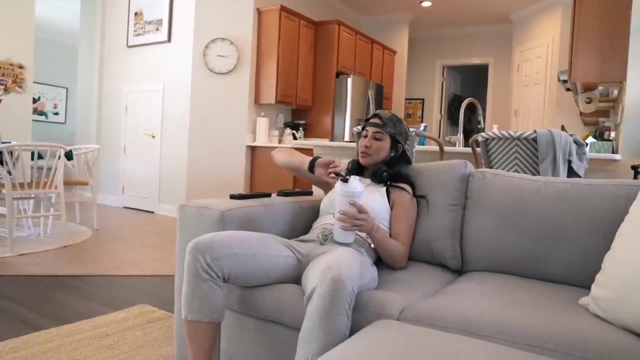 a high-quality, high-leucine protein supplement, such as so-called vegan whey, which combines pea and brown rice protein to give it a similar amino acid profile to whey protein. Many people still believe that if you don't eat protein within 30 minutes after training, your entire session was. 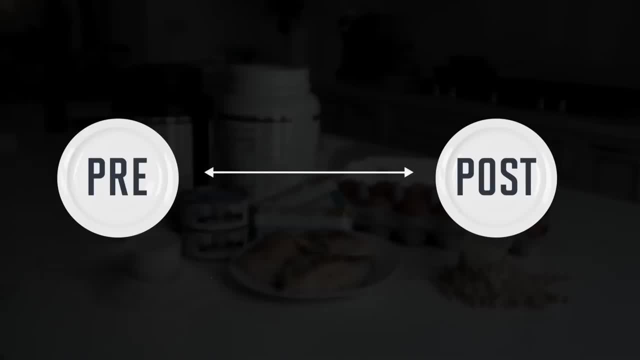 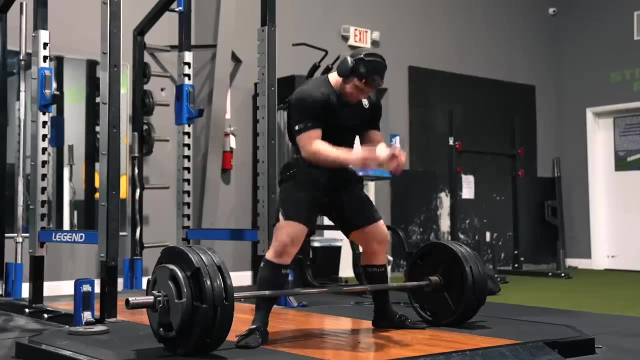 wasted, But this idea was debunked years ago. In reality, as long as your pre-workout and post-workout meals are within roughly four to six hours of each other, you'll be maximizing the anabolic response to training. A possible exception to this. 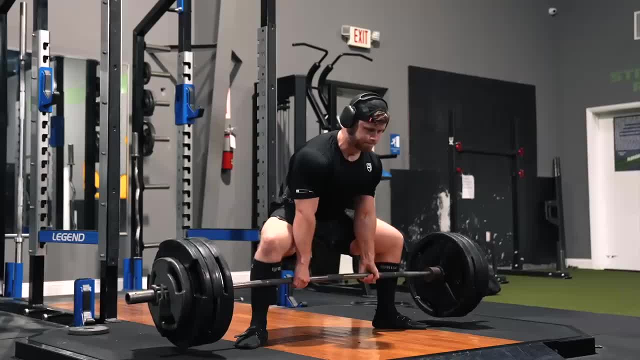 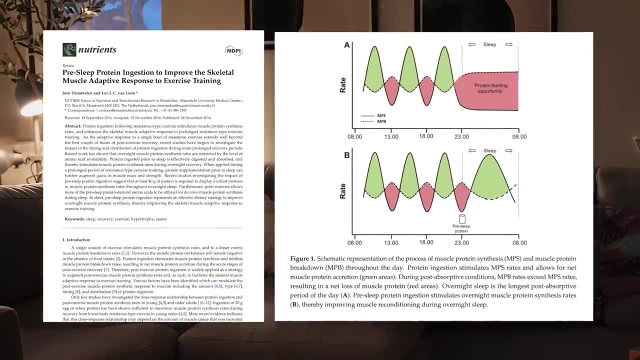 would be if you train fasted, in which case you should try to consume some protein as soon as you can after your workout. Perhaps a more important but less discussed timing variable is consuming protein before bed. This study from my friend Joran Tromelin and his colleague Luke Van Loon 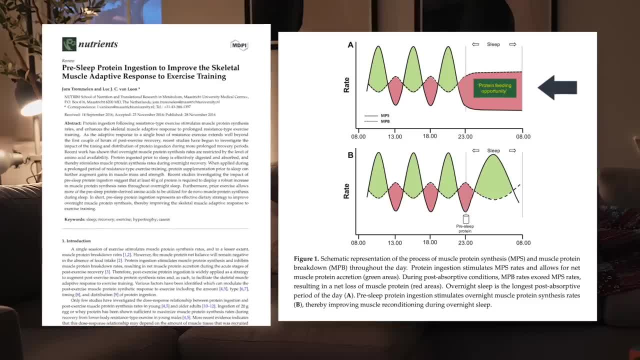 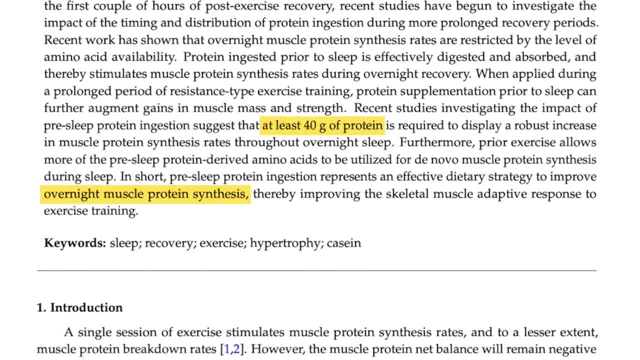 described pre-sleep protein as an important protein feeding opportunity. They suggest consuming roughly 40 grams of protein before an overnight fast to improve overnight muscle protein synthesis. This is personally what I aim for, Granted two other longitudinal studies that directly tested consuming a slow-digesting casein protein. 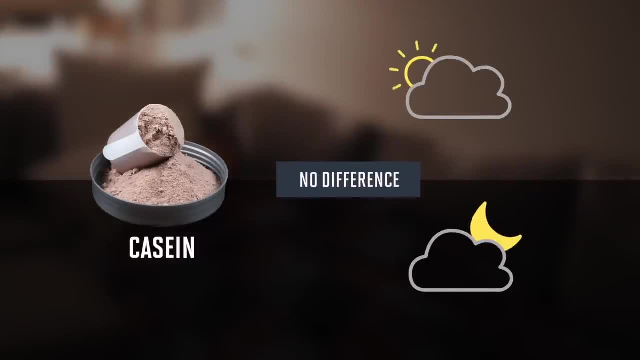 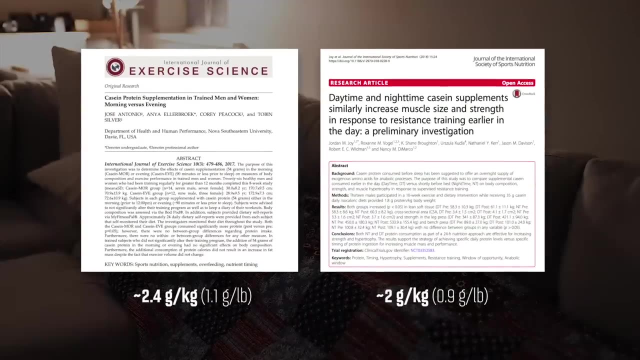 either before bed or in the morning, found no significant difference after eight to ten weeks. However, both of these studies had subjects consuming a very high protein intake overall, in the range of two grams per kilo, or about one gram per pound, once again highlighting that, as